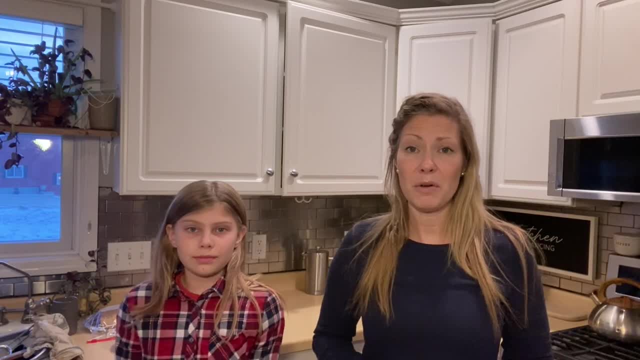 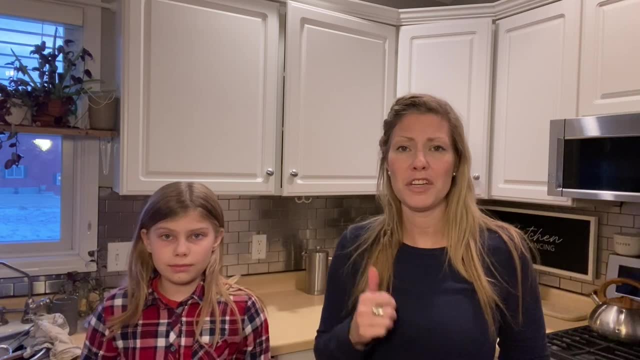 craft cupboard. We get it out whenever we need it. Actually, it's also a really nice stress reliever when we have kids working at screens. Just have something to poke or squish when they're sitting there. It just seems to be a really nice stress reliever. So we are currently all out of colored 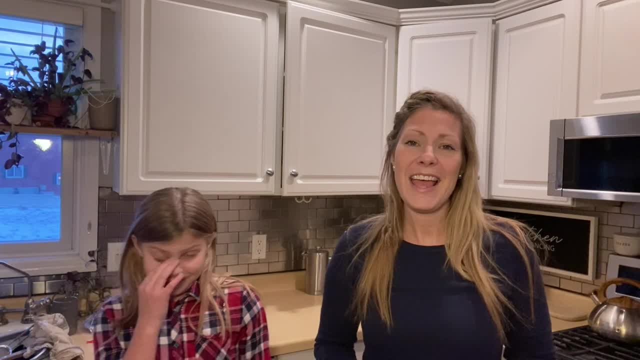 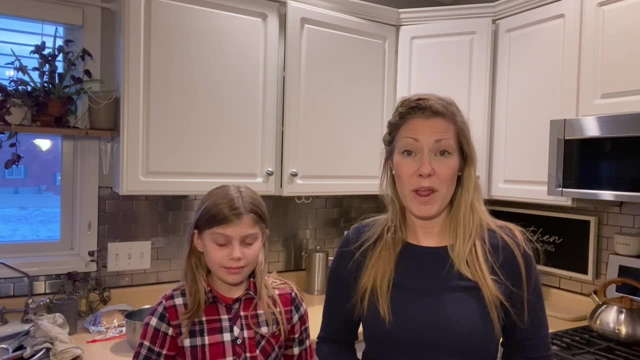 dye because we're doing a lot of slime projects lately, but we decided we're going to make it work and make some snope play-doh today. So we're going to make some white play-doh and I'm going to show you how we make this soft. 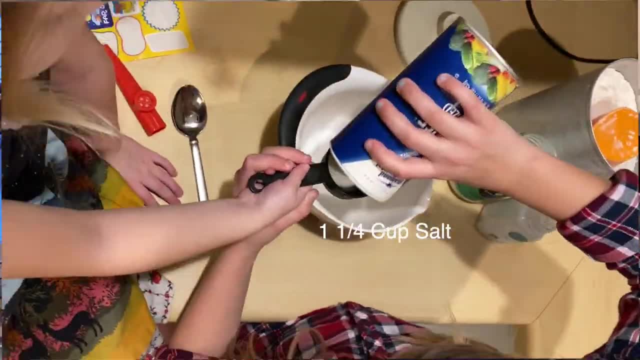 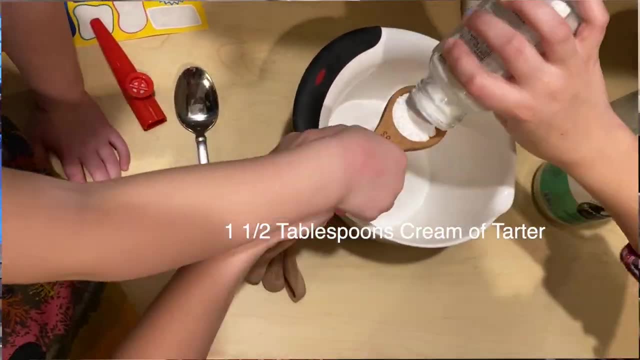 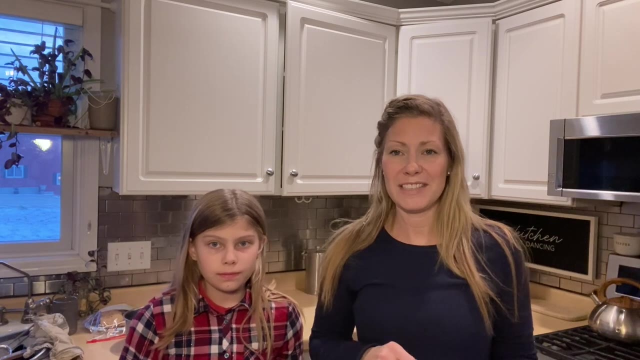 play-doh. So we are going to add one and a fourth cup of salt, Then we're going to add one and a half tablespoons of cream of tartar, So that cream of tartar might be one of those little ingredients that you may or may not have in your cupboard. You do because we like to make whatever you make. 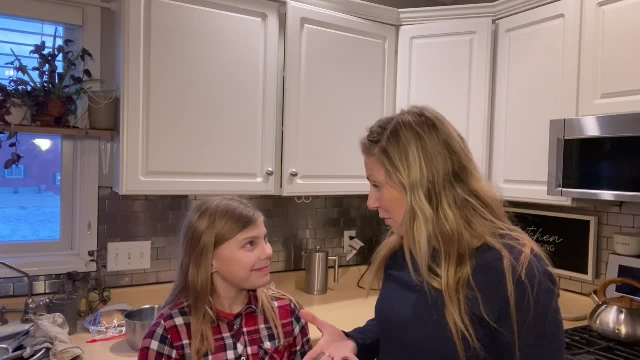 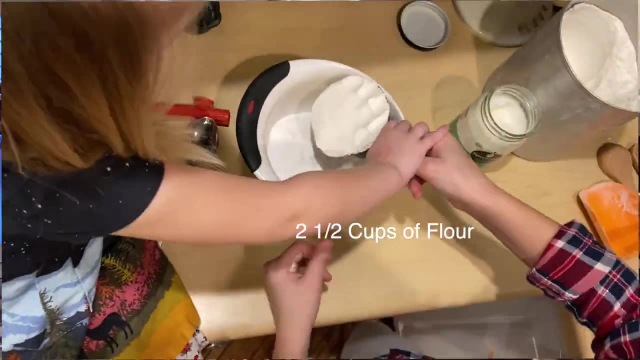 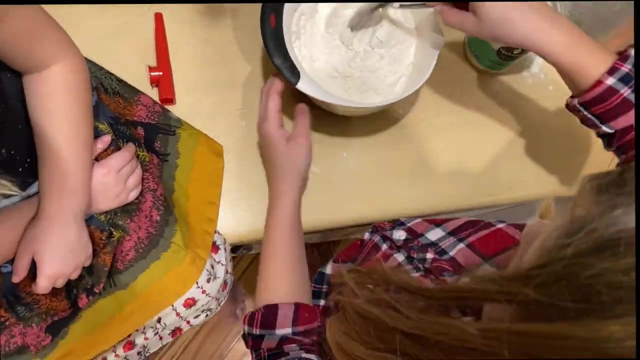 with cream of tartar. What kind of cookies do you guys love? Snickerdoodles. So we make snickerdoodles and we use cream of tartar for that And two and a half cups of flour. So we're just adding two and a half cups of water to a pot. 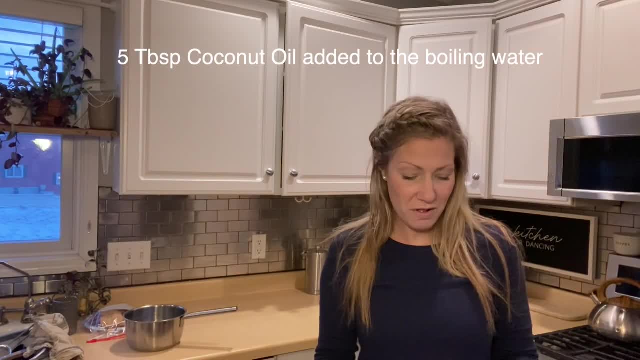 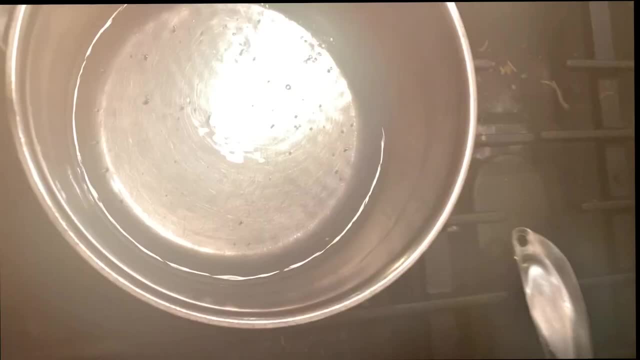 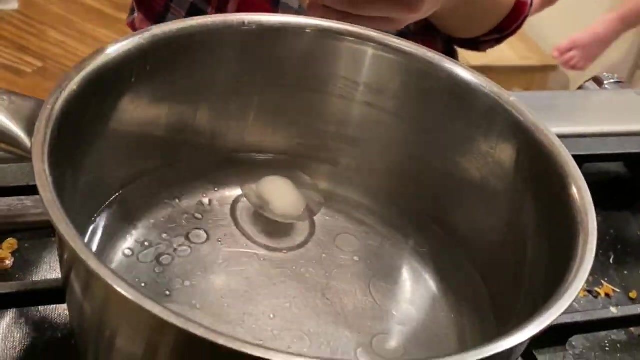 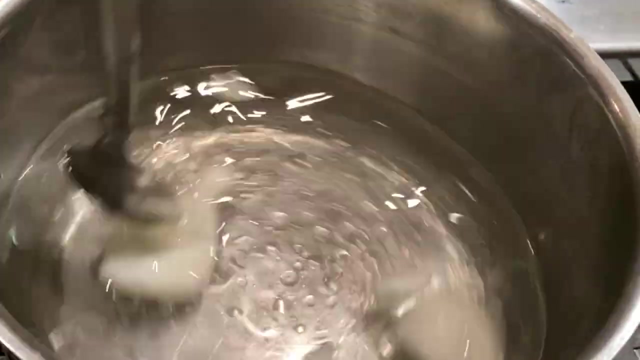 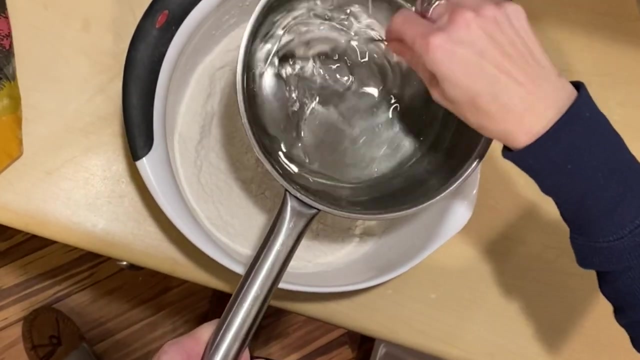 Also, we need five tablespoons of coconut oil. Bring your water to a boil. We're going to turn our boiling water off and we're going to add five tablespoons of coconut oil to this. All right, so this is the job for an adult, Once our hot water and our coconut oil is melted in. 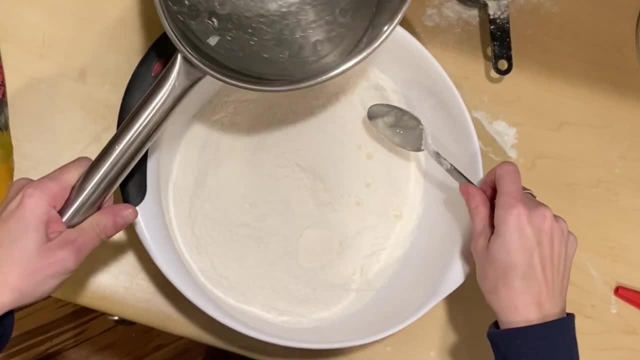 that hot water. we're going to bring that to a boil, So we're going to add five tablespoons of coconut oil to this. We're going to turn that over and pour it into our flour mixture And we're going to stir all of this in. 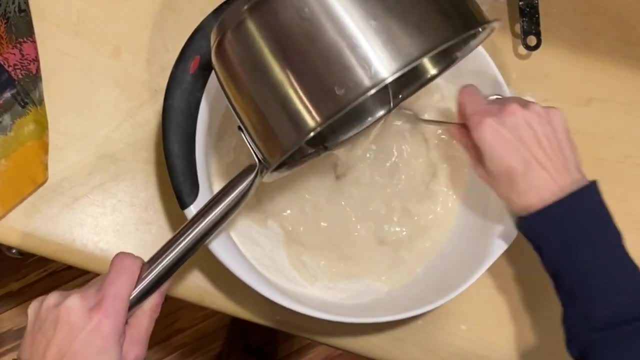 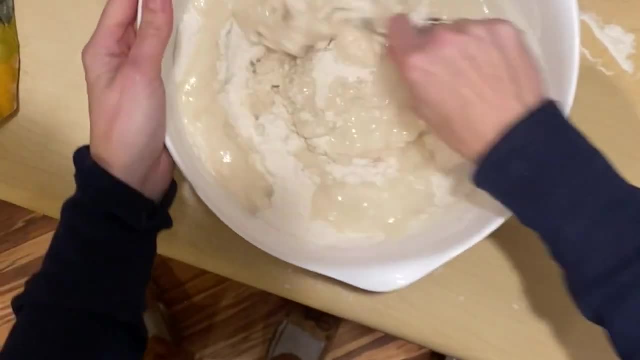 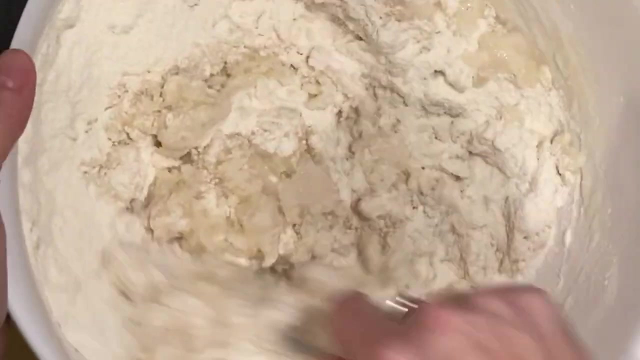 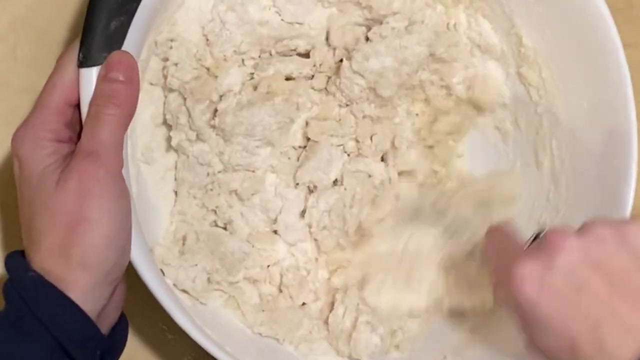 And this is going to form our dough Now. at this point we could add food coloring or any other natural colorings. You could also add some essential oils if you wanted it to smell differently. I kind of just like it plain, and we're just going to call this a. 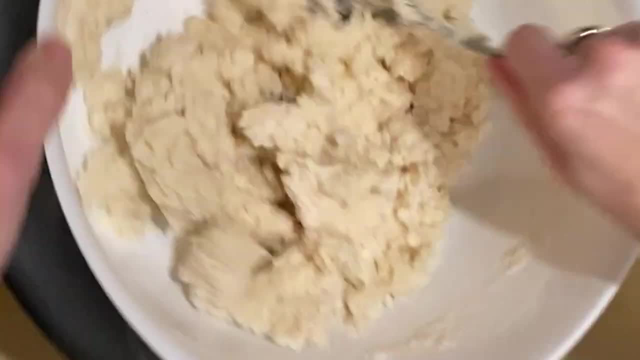 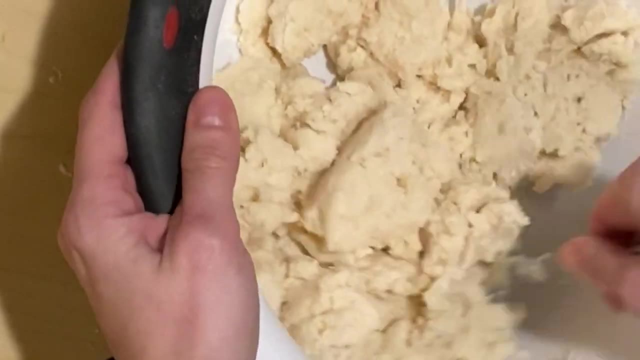 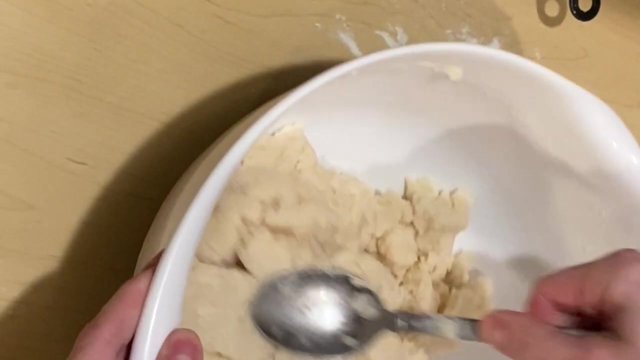 Snow Play-Doh Right kind of reminds me of what we're gonna do next. We're gonna be making some bread next. We're all out of bread in the house. We need to make some bread. We're gonna let it cool a little bit before we start playing with it, because we do have some hot boiling water here. 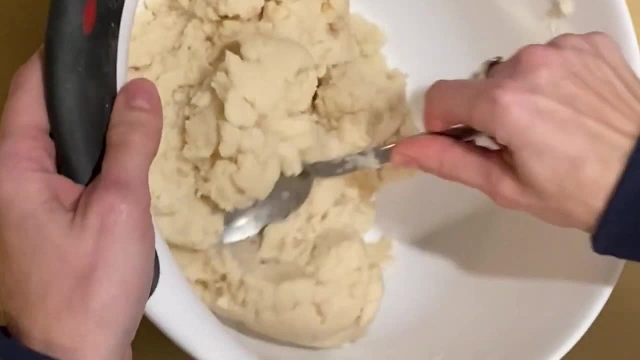 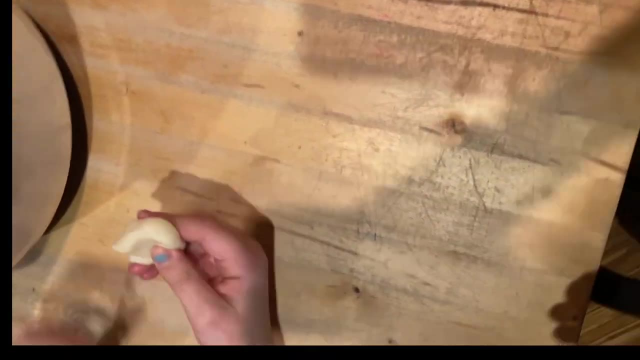 So we want to be careful, especially with little hands on this, before we start kneading. Okay, so once we've let it cool a little bit, then it's cool to start kneading it, Forming it into the inevitable shape that it will be in. 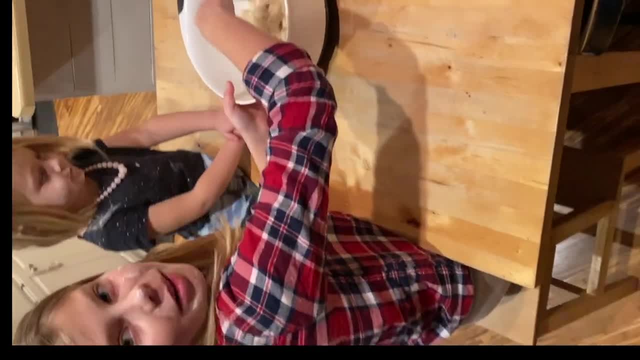 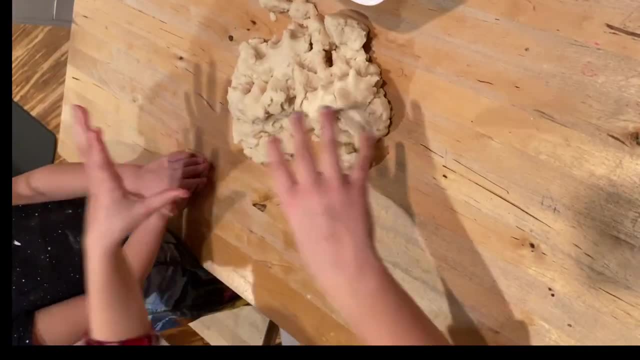 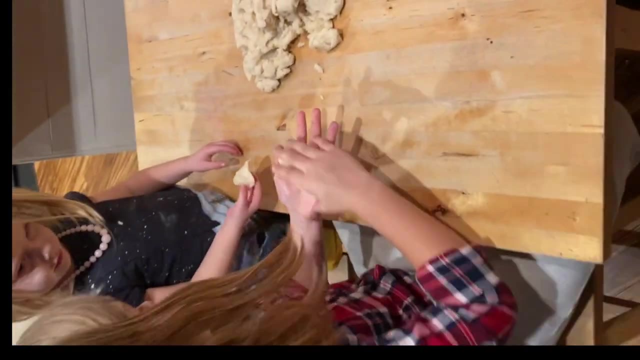 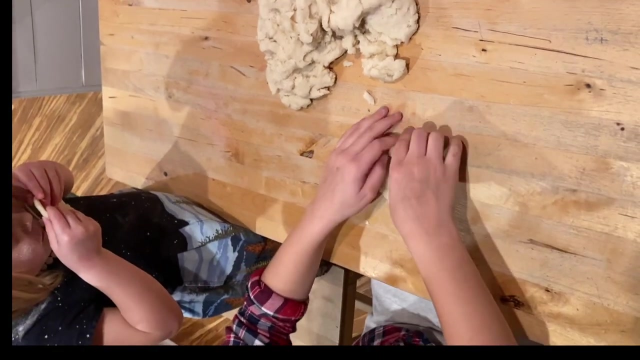 Isn't it lovely? There's enough to share, which is nice. if you did have, If you did have, colorings that you wanted to add, now would be a good time to divide this up and Make some colors out of it. We also just keep this either in a ziploc bag or an airtight storage container to play with. 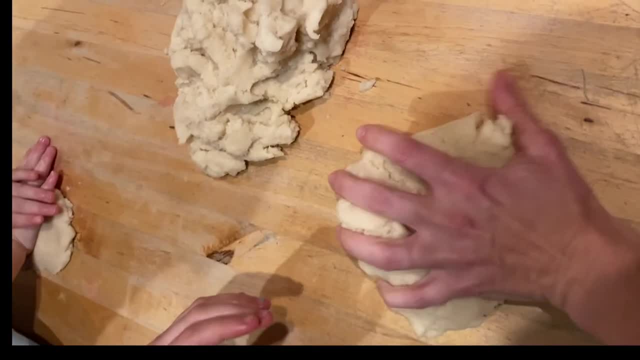 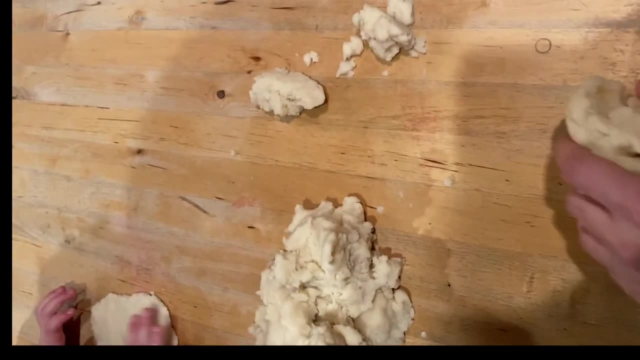 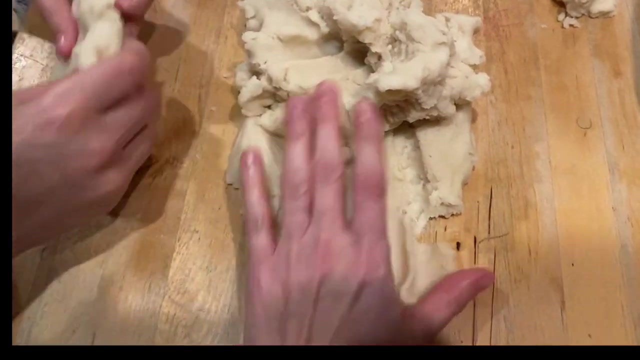 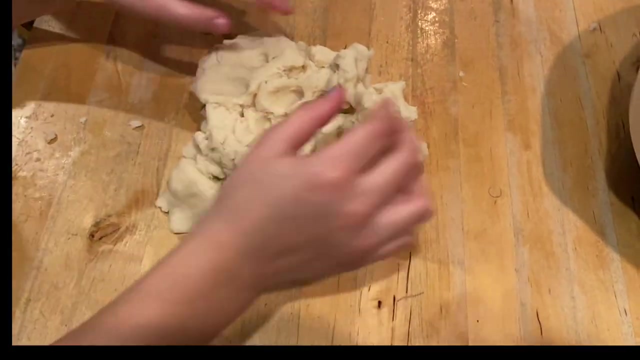 Nothing better than a fresh batch. Oh yeah, you can't collect even no, I don't know how nice and soft. that is big and there's a lot. there's a lot of it, which is nice because so we can divide it up amongst all of you guys. 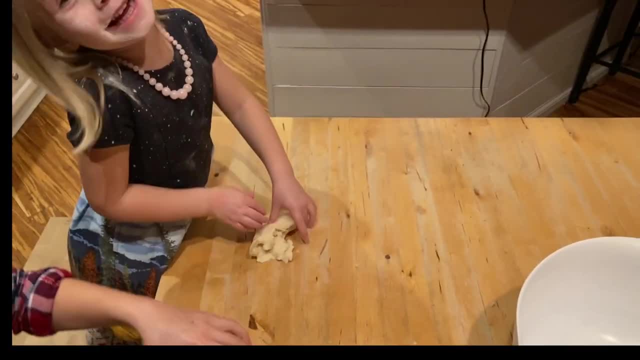 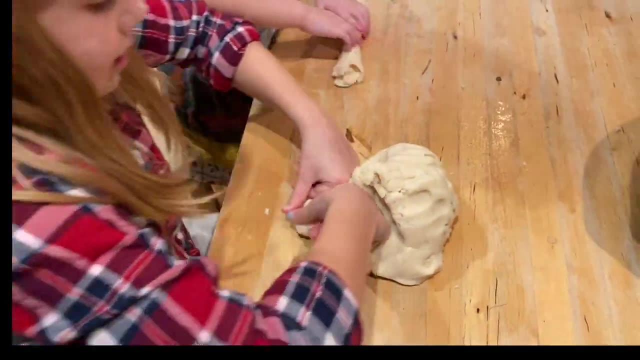 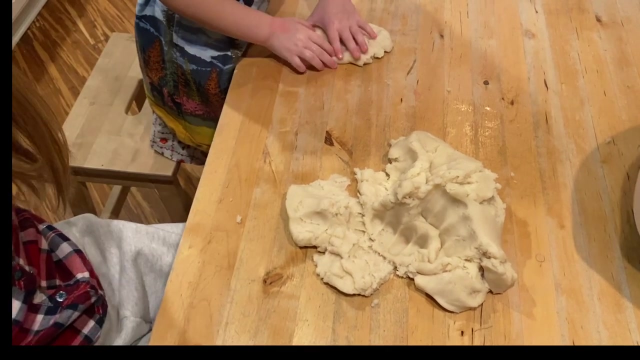 This is so much fun, Mom. Thank you, Mama. Hey, you gotta knead it. There you go, just like our bread. There you go, Mom, there's the bread. No, come on, Come on, Smells actually really good. 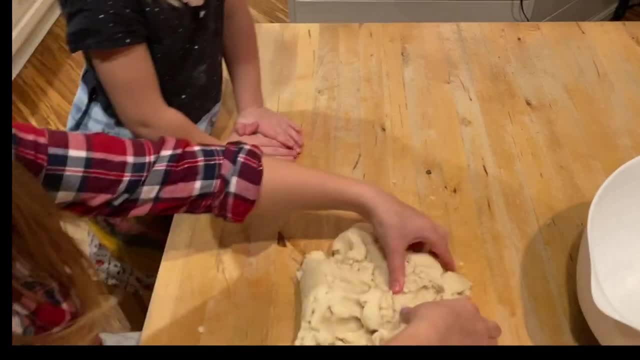 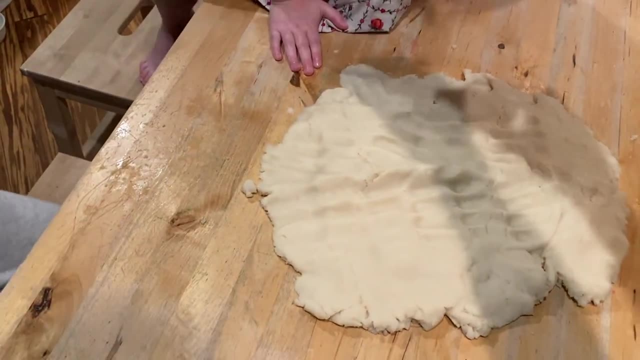 Smells good. Smells pretty good. We do have a little bit of grapefruit essential oil, so we're going to drop just a few drops on this and then let them mix it in. All right, so don't touch the oil itself. 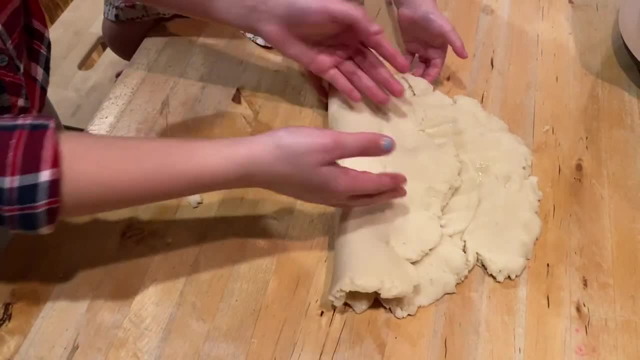 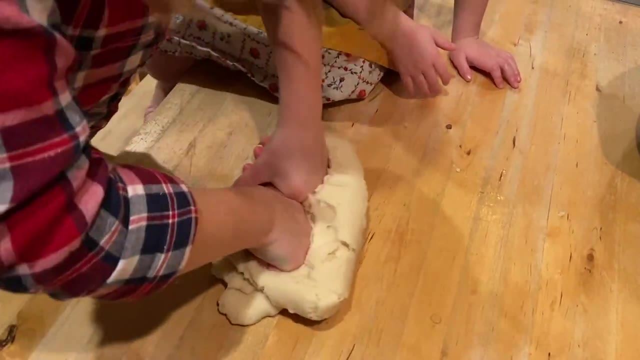 but fold that in, Otherwise the oil will stay on your hands. Squish it in yep, knead it in. You could add any scent you'd like. You don't have to add it in. You don't have to add anything.